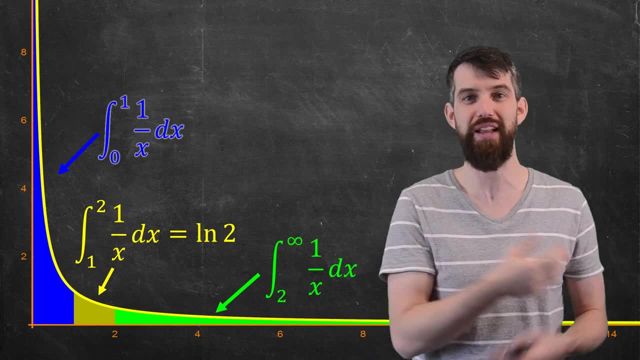 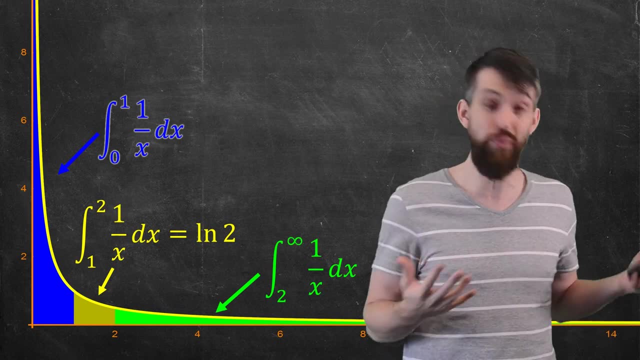 Or when we're setting our domain of it to be going all the way off to infinity. how is that defined? And then, are these positive numbers? Are they going off to positive infinity themselves? You might think. well look, there's two different infinities. 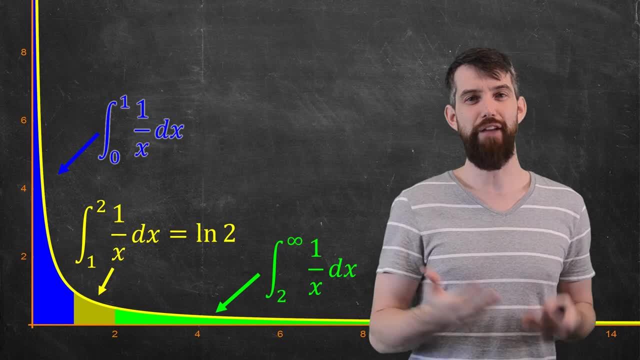 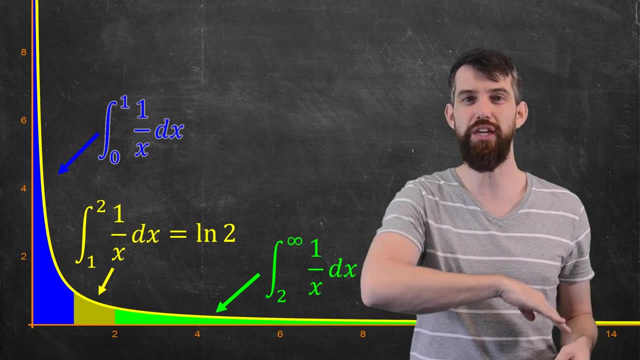 Both of these areas are both infinite. But if you recall, when we were doing limits, back in Calculus 1, there were all kinds of functions like, say, arc tangent, where the function was increasing, increasing, increasing, but it would level off. 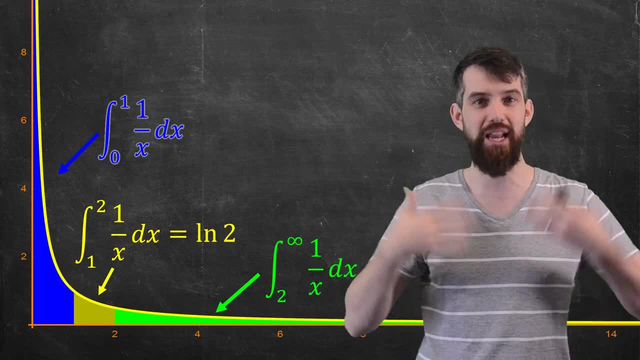 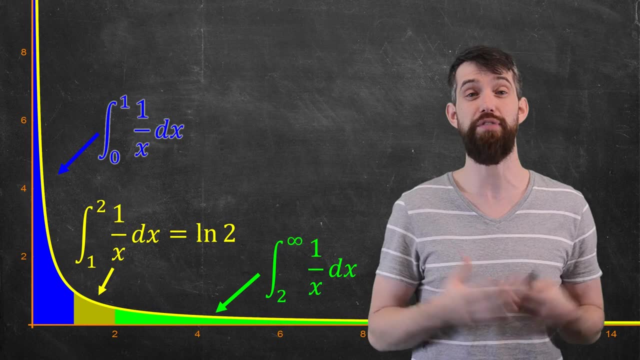 So in this integral from 1 to infinity, yes, the area is getting bigger and bigger and bigger the further you go off to the right, But does it converge in some value Or does it really go and stretch off to positive infinity? So we need to make precise these concepts and compute the values if they do indeed converge. 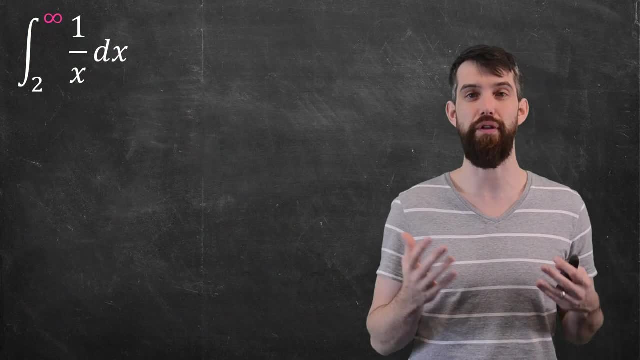 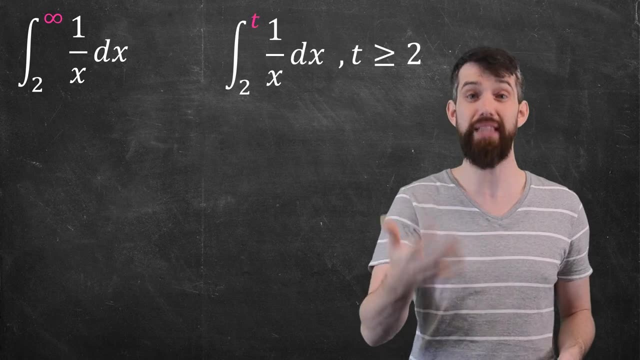 So let me focus on the 2 up to infinity integral first. The thing that's problematic for me is the infinity side, So what I'm going to try to do is consider something slightly different, That is, the integral of 1 over x, but not from 2 to infinity, 2 to some t value. 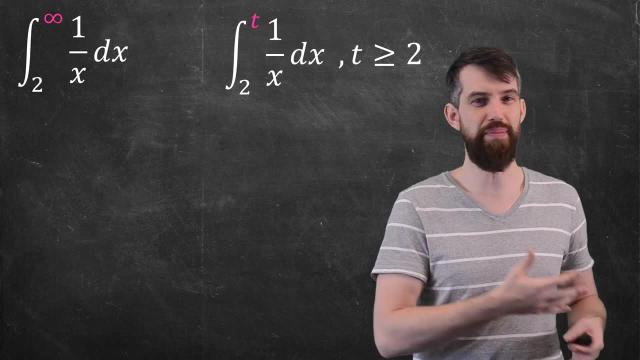 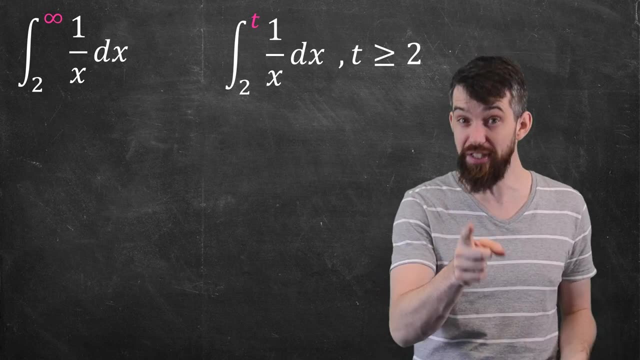 where t is just a number that's greater than 2.. I'm thinking that t here might be 7, or 100, or a million or a trillion, but it's always a number, And if it's a number I can do this integral. 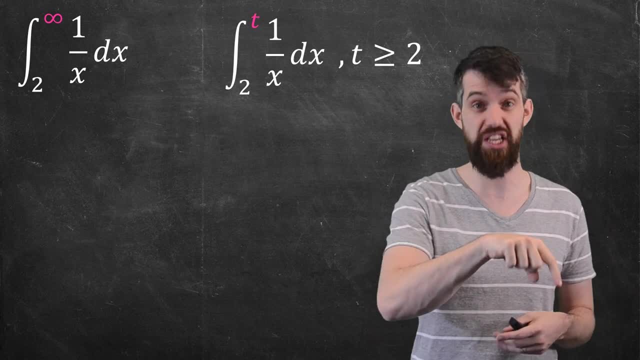 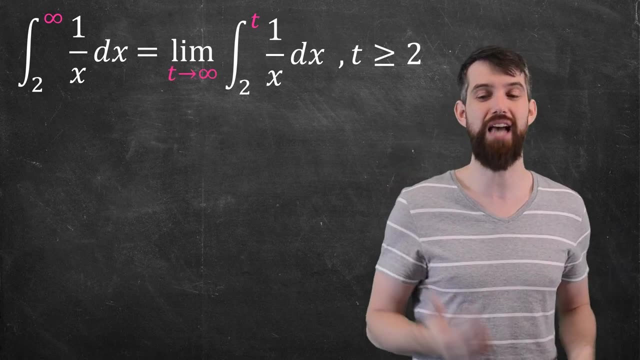 So this integral is actually a function of t. For every input t, you get a different number out of it, And if it's a function of t, I can take its limit as t goes to infinity. So that is how I'm going to define the so-called improper integral, from 2 all the way up to infinity. 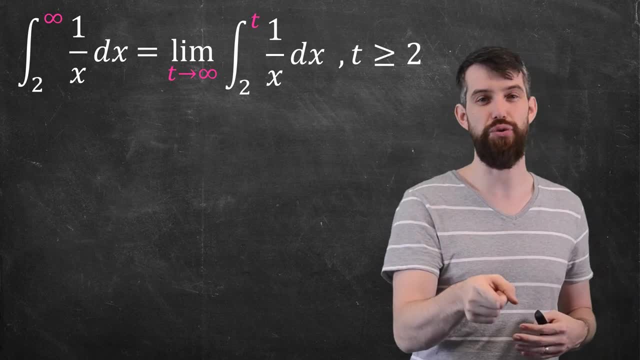 It's 2 up to t, where I then take the limit as t goes to infinity. Why is this helpful? I'm not going to touch the limit sign for a moment, I'm just going to do this integral with this arbitrary t there. 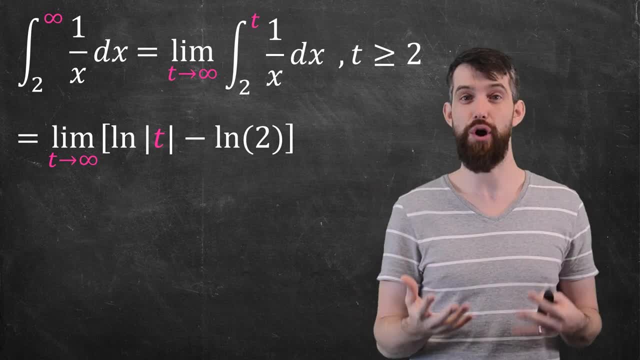 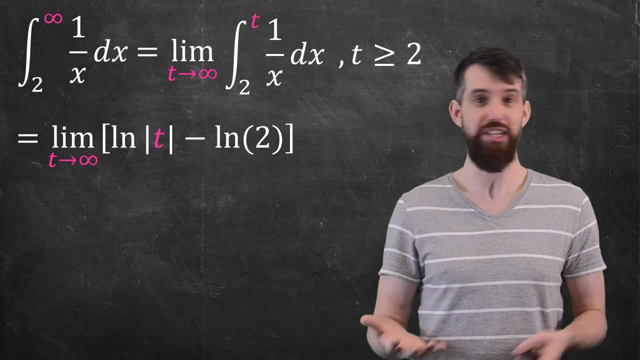 And this is straightforward: It's the logarithm of t minus the logarithm of 2.. And now this is just some function, and I am asking what some limit of some function is. Well, it just depends on what logarithm looks like. 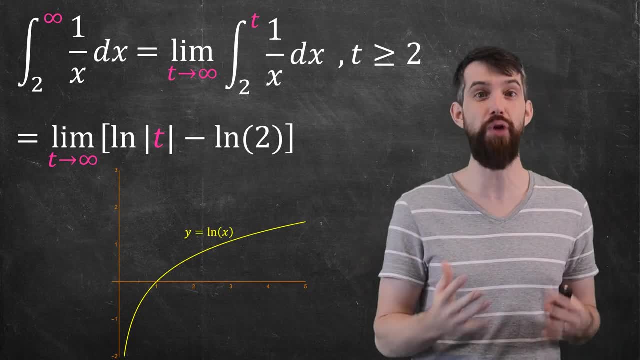 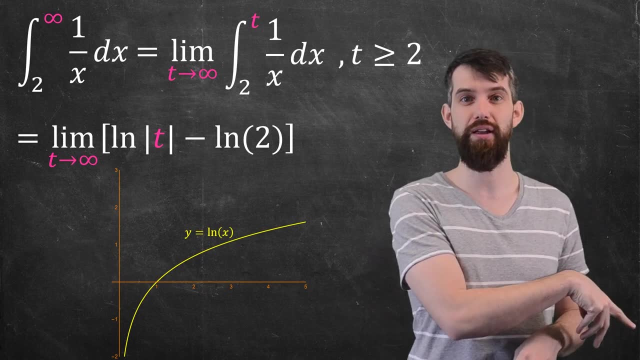 So here's what the graph of logarithm is, And you'll notice about this is that if t goes to infinity, then the logarithm is also going to go to infinity, And so, as a result, this thing is just equal to infinity. 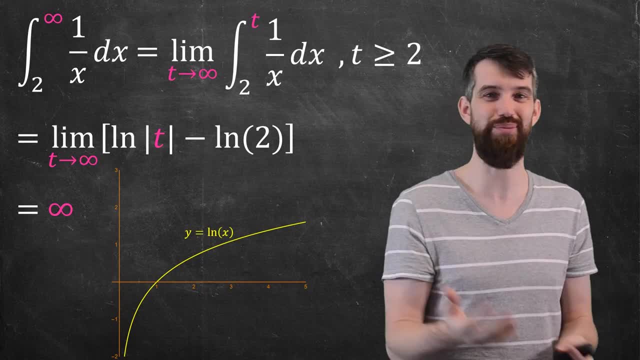 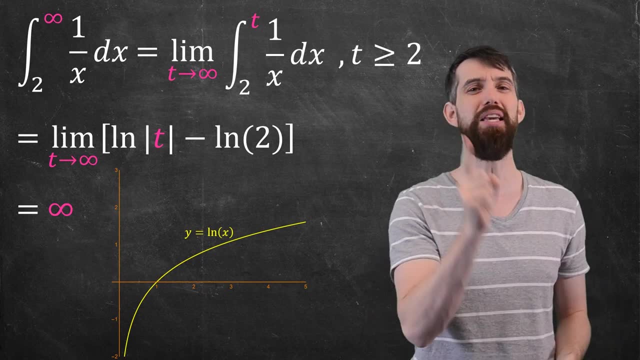 Okay, you might be telling me this is kind of silly. It was going off towards infinity. The answer is: infinity is sort of what you expected. Am I really doing anything with all of this? Well, let me give you a different example. 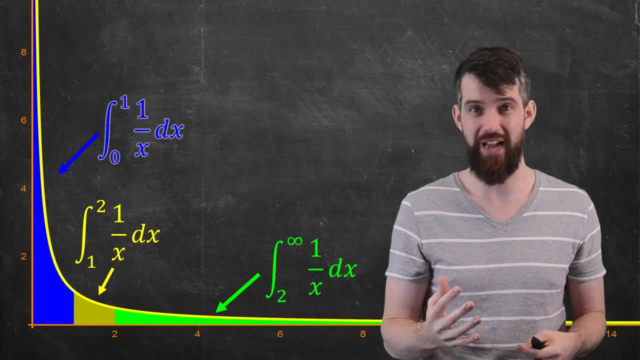 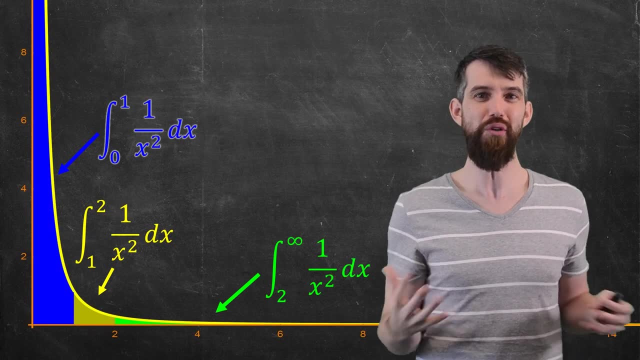 Remember we were focusing on the green region here. for 1 over x. But let me change the function just the tiniest little bit. Let me make it 1 over x squared now And for 1 over x squared, because the x squared is bigger than x. 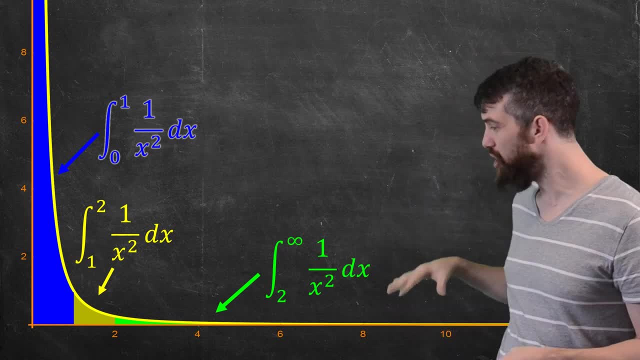 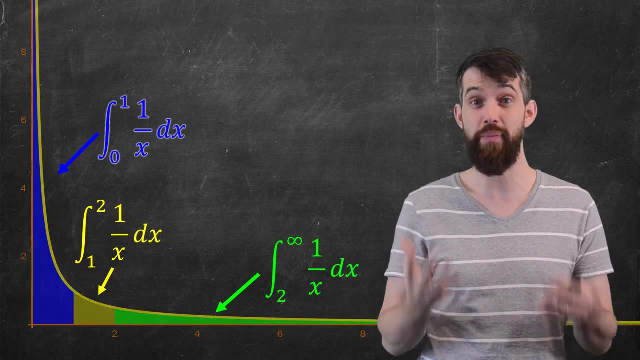 I'm dividing by it. What really happens is that the green region got a bit smaller And the blue a little bit bigger. Let me go back. So this is 1 over x. You see, the green region is a little bit bigger here. 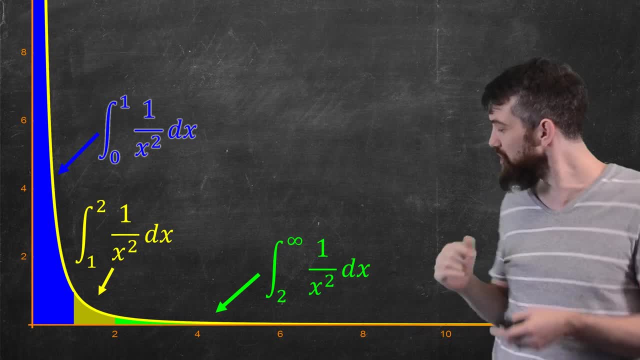 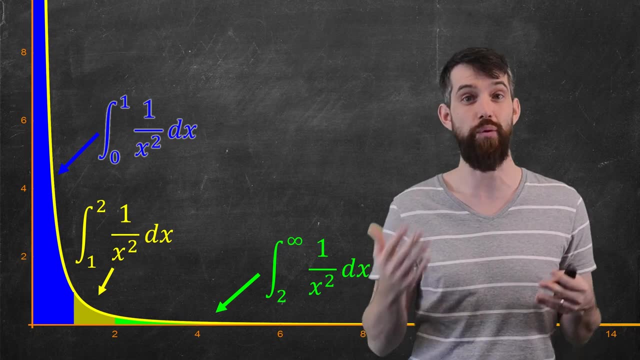 And now if I go to 1 over x squared, it compresses faster and the green region is a little bit smaller. The original for 1 over x goes to infinity. But what about for 1 over x squared? What happens there? 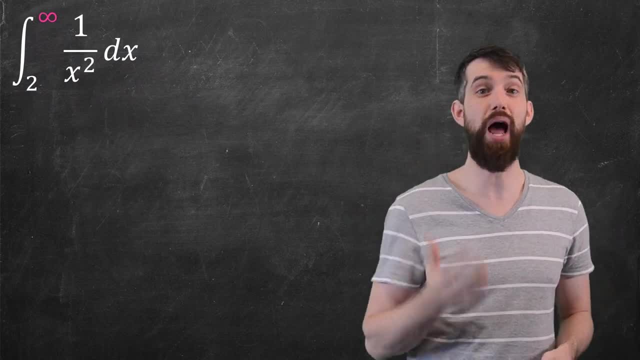 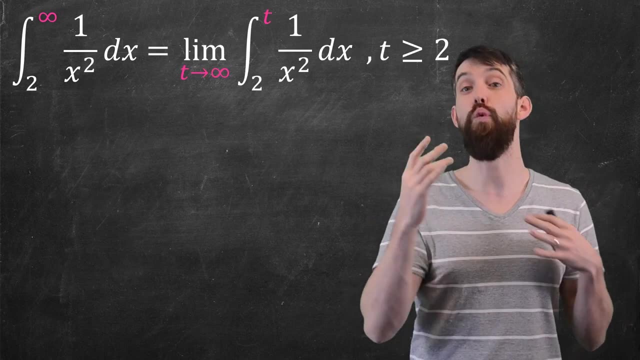 So if I focus in on that integral, I'm going to apply my definitions just as I have before. Well, this is the limit As t goes to infinity. the integral from 2 up to t of 1 over x squared dx. 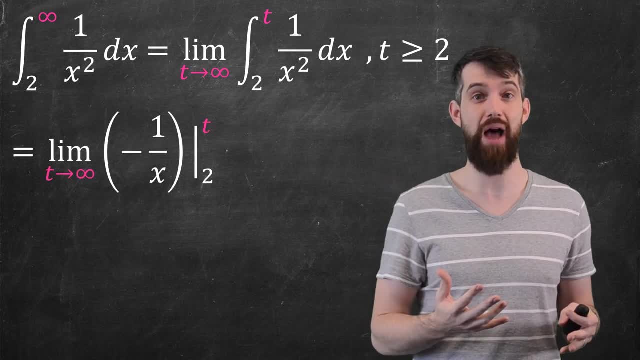 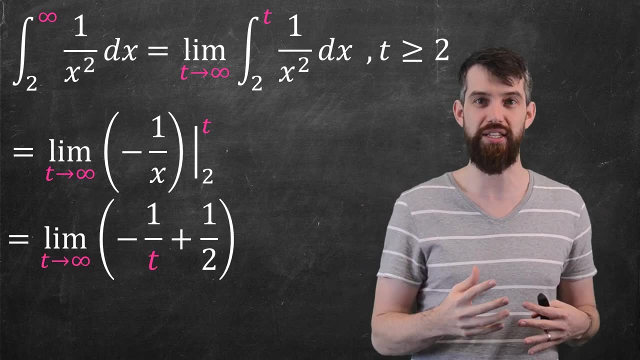 1 over x squared is something I can do, So I'll leave the limit out the front And I just get an antiderivative of minus 1 over x between 1 and t. I evaluate that And so I get minus 1 over t, minus minus 1 over 2.. 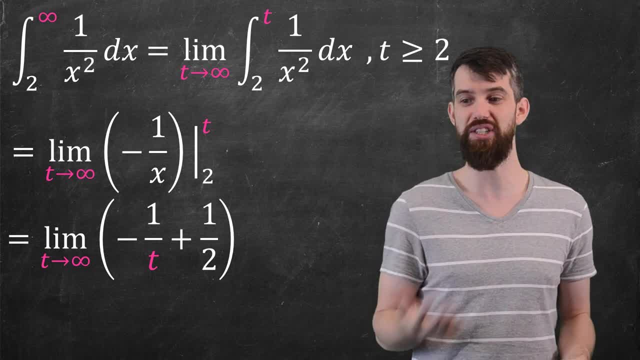 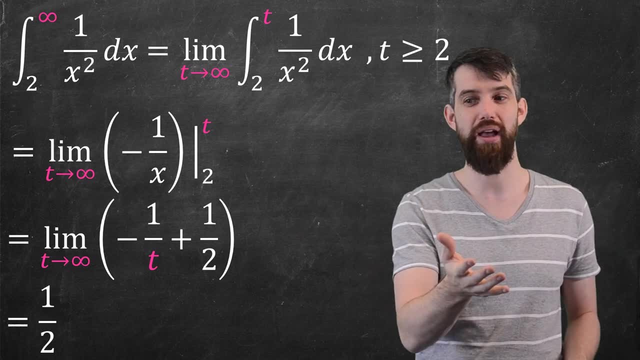 And now I can do this: If I plug in t to infinity, 1 over infinity is just going to go to 0. But that 1 half that we still have here, it doesn't go away. So this, indeed, is just the value 1 over x. 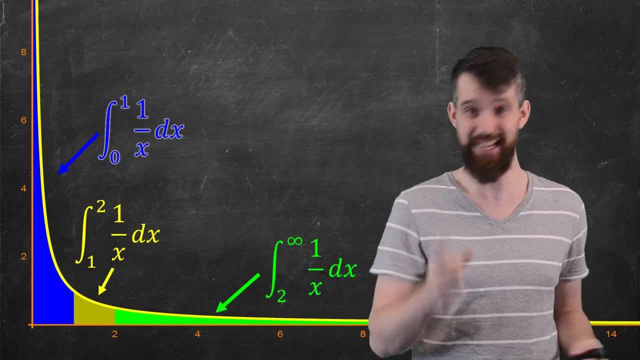 1 half. Okay, so that's the green ones. That's going off to infinity. That's our case 1.. What about case 2?? In case 2, we're talking about these integrals from 0 to 1. 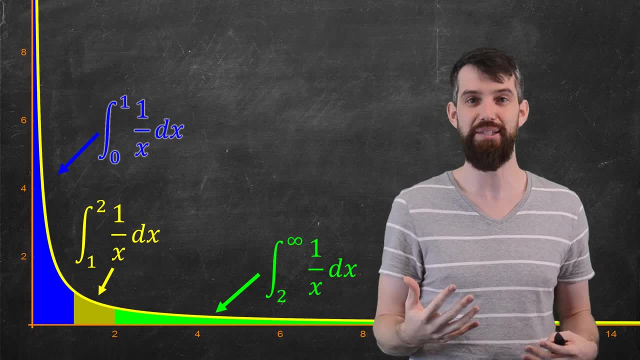 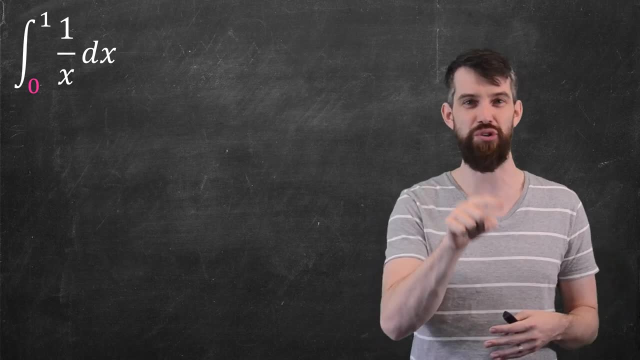 where I have a discontinuity, I have a vertical asymptote at 0. So let's focus on that particular interval. I want to do the same sort of trick: Replace it with a t instead of a 0, because 0 is my problem spot. 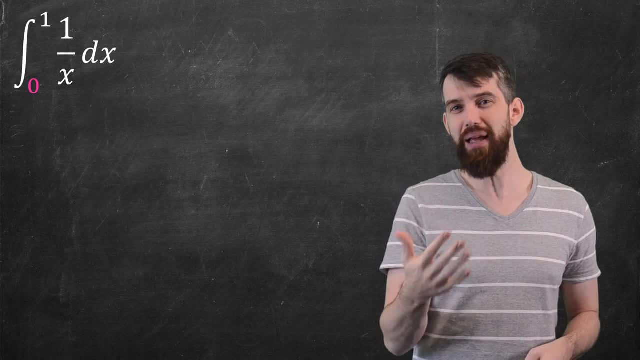 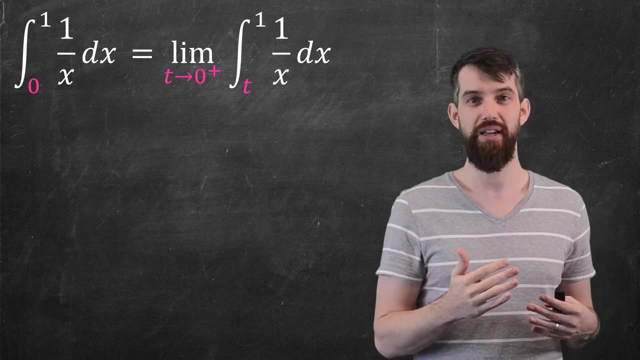 0 is my spike to infinity. But now my limit is not going to be when t goes to infinity, It's when t goes to 0. And in particular, when t goes to 0 from the right. So instead of having 0 to 1,. 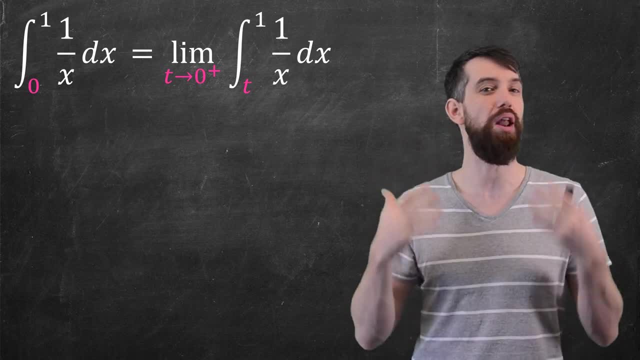 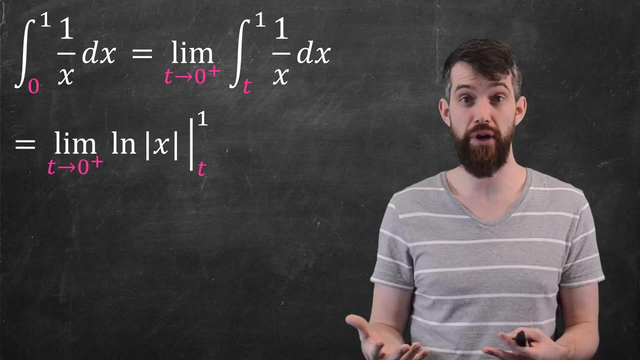 I have t up to 1.. And I imagine t is a number like 0.1, 0.01, 0.001.. Again, I can leave the limit off the right-hand side and I can compute this: The antiderivative or an antiderivative of 1 over x. 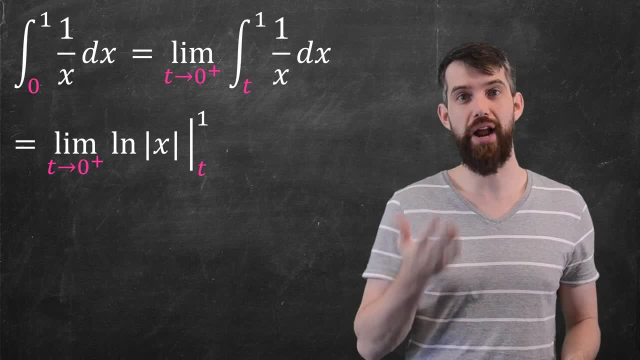 is the logarithm of the absolute value of x. I plug in 1 and I plug in t, And what do I get? Well, logarithm of 1 is 0. So I'm just subtracting off the logarithm of the absolute value of t. 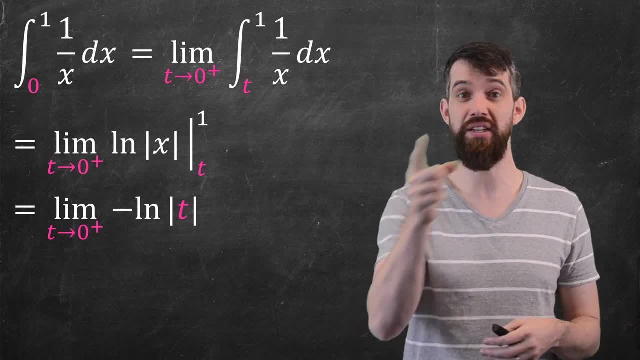 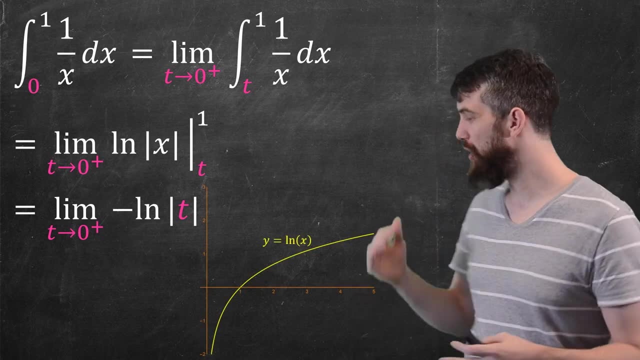 Well, what's logarithm of t when t is going to 0 from the right? Well, what's our graph of logarithm? There it is once again, And you'll notice about logarithm that it has this vertical asymptote at 0.. 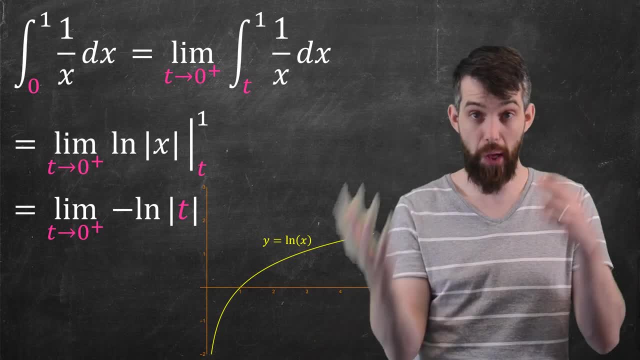 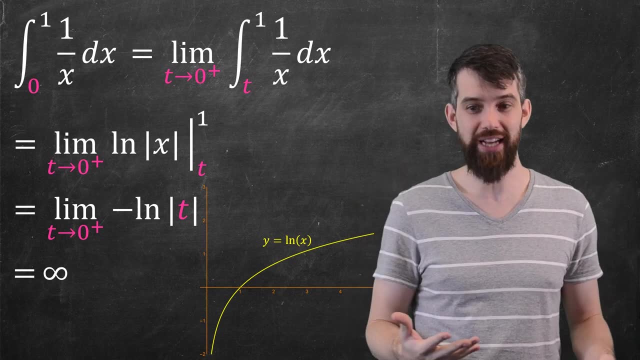 It goes down to minus infinity. Well, because it's minus, the logarithm of this minus, minus is positive. So again, this is going to go to infinity. So for the function 1 over x, we've seen that, the blue region as well. 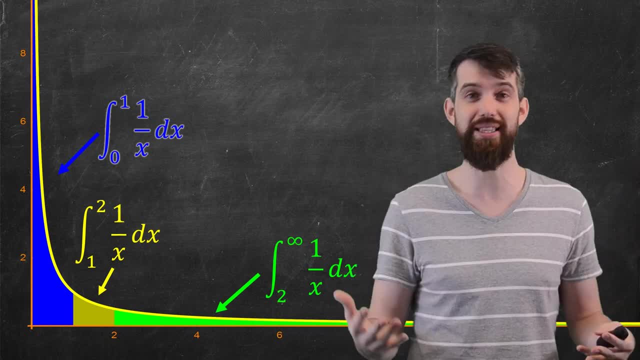 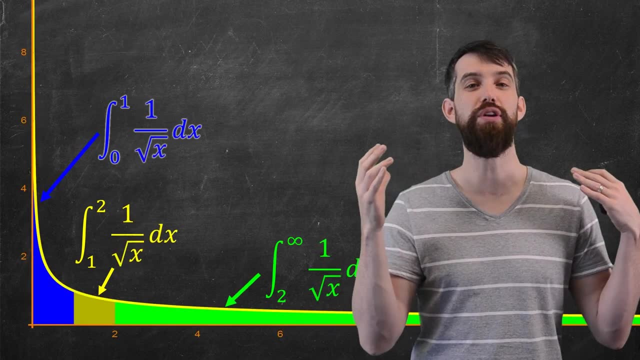 also is going to go to infinity. Well, is that always the case? Again, it's not always the case. Okay, so let me give you a new example. Instead of 1 over x, I'm going to give you 1 over square root of x. 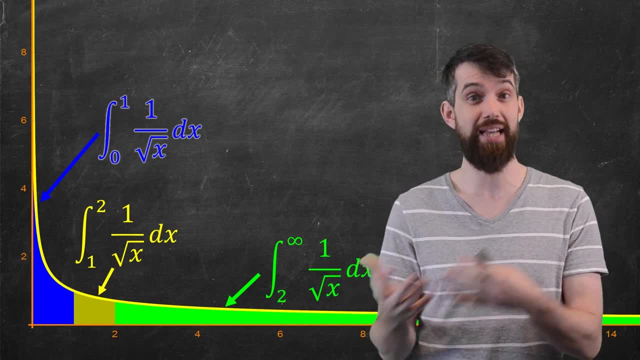 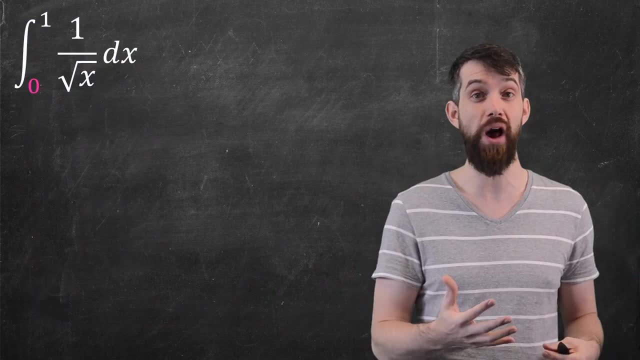 1 over square root of x grows more slowly as x goes really large. So now the green region is bigger and the blue region is smaller. Okay, so let's focus in on the blue region. the integral from 0 to 1.. 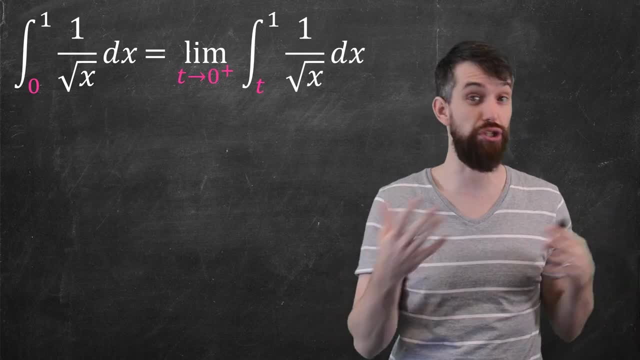 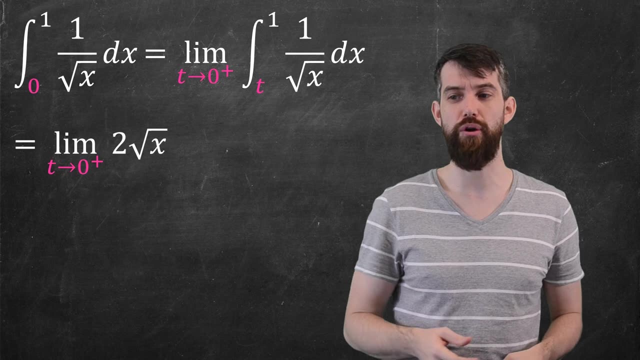 I know how to do this. now It's going to be the limit, as t goes to 0, from the right of the integral of t up to infinity of 1, over root, x, dx, And I know how to do this: integrand It's just going to be a power rule. 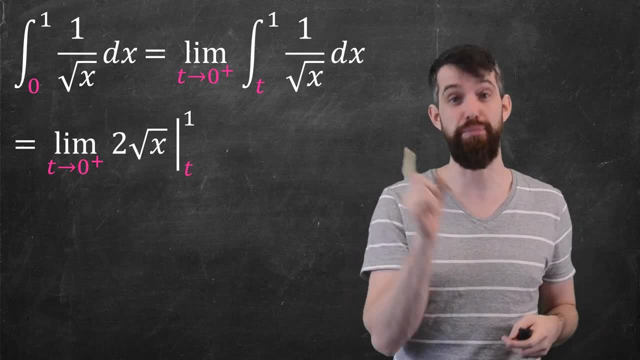 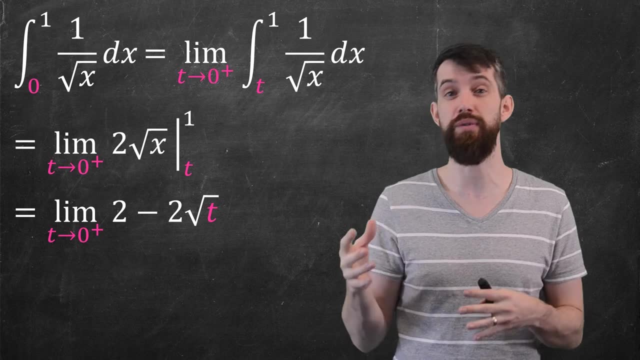 So I leave the limit out the front, The limit of 2 times root x, and I'm evaluating between t and 1.. If I plug those values in, I'm going to get a 2 minus 2 root t. Now it's just a question of doing the limit. 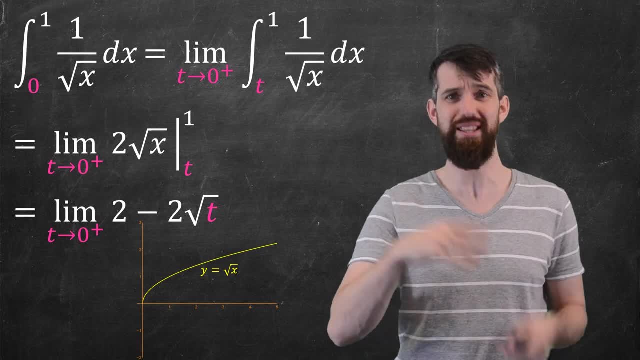 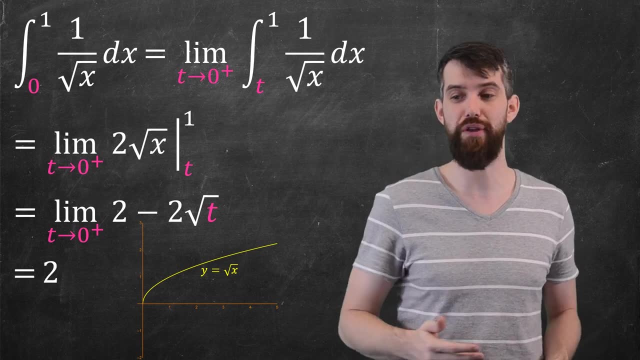 I'll remind you that the graph of root x looks like this, as you send this value to 0. You consider root t as t goes to 0. You just indeed get 0. So that leaves behind only the 2 at the front. 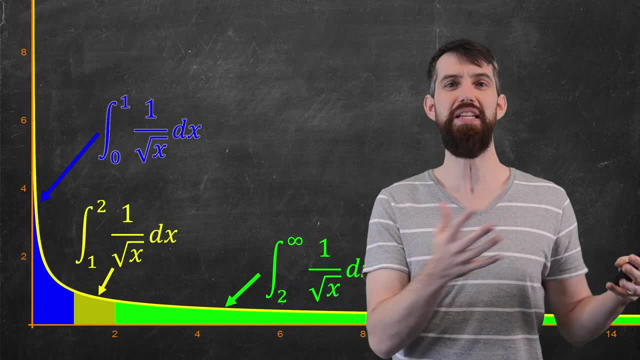 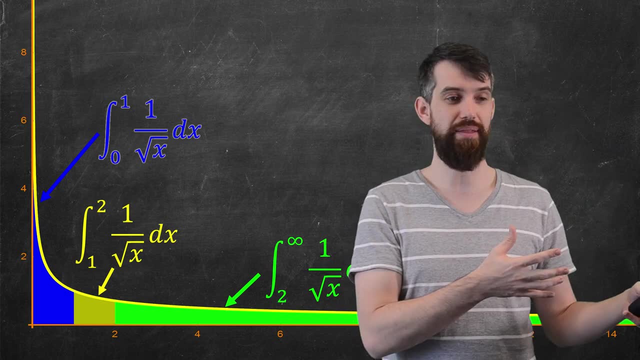 and so this value is 2.. So what we've seen in these examples is that for either case 1, which is when you have one of the bounds of integration being infinity, that that may or may not converge to a finite number, or it may diverge to infinity. 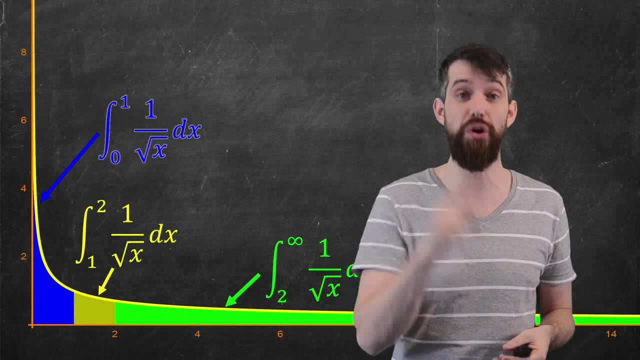 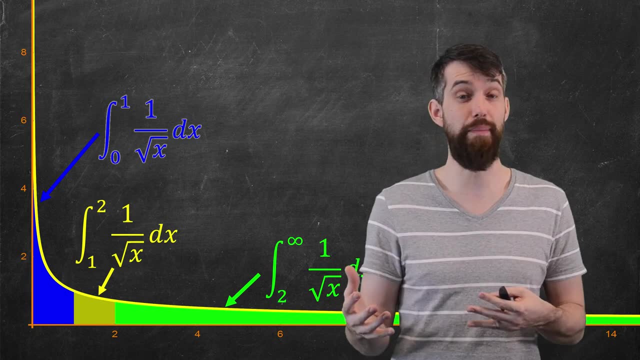 And likewise when you have a vertical asymptote, so a discontinuity, a spike to infinity, a 0 in the denominator. again, you can do a very similar trick with a limit, And there again it may converge to a number or it may diverge. 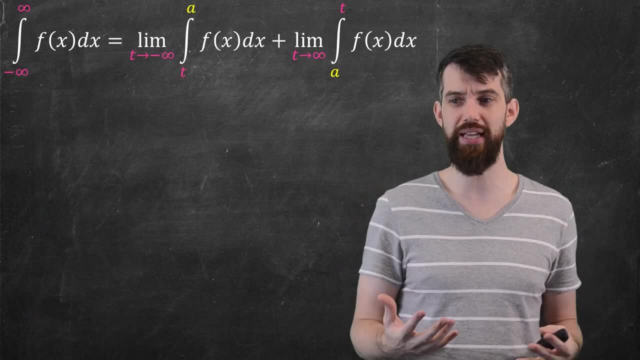 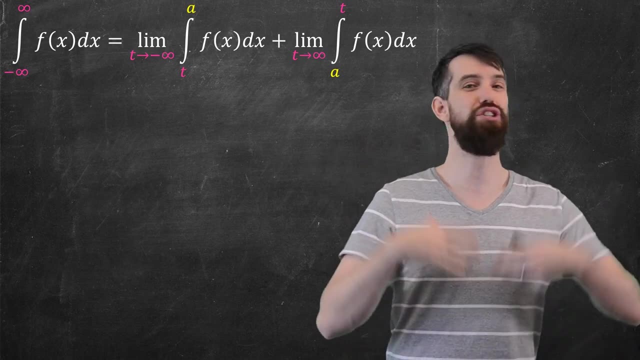 Finally, I want to talk about the sort of more general case. If I take the limit from minus infinity all the way up to infinity, so I'm doing it on both sides. well, I just do a sum, I just choose some random value. 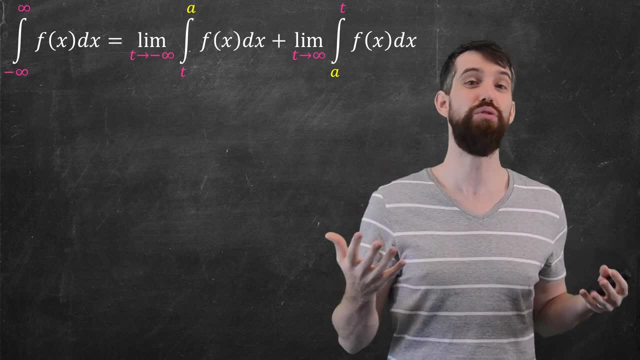 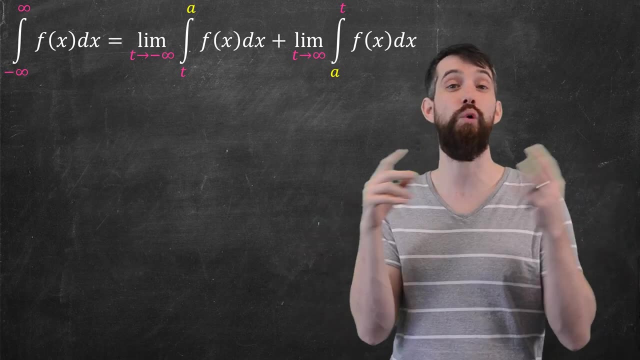 in the middle like a, and then I do an integral from t all the way up to a and from a all the way up to t, and then I take those t values either to minus infinity or plus infinity. I can do both sides of it sort of separately. 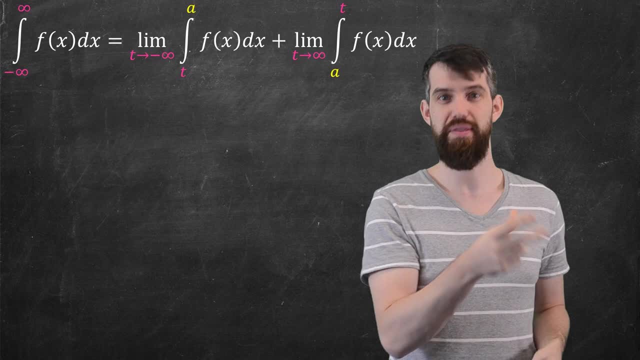 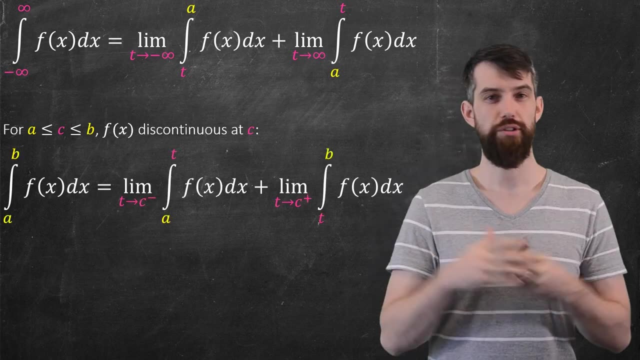 when I break it up at some middle point a, And then likewise if my point of discontinuity is somewhere in the middle. so my c is my problem spot. so then what I can do is take this integral from a up to b and I break it up. 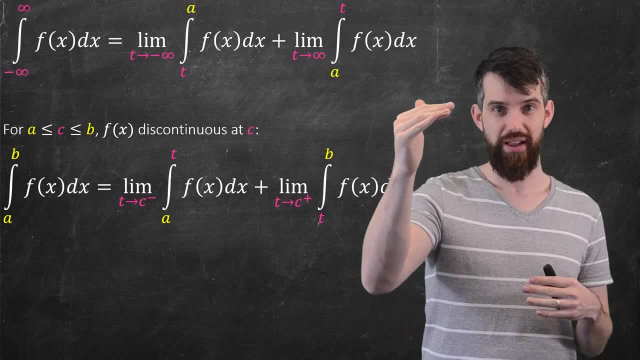 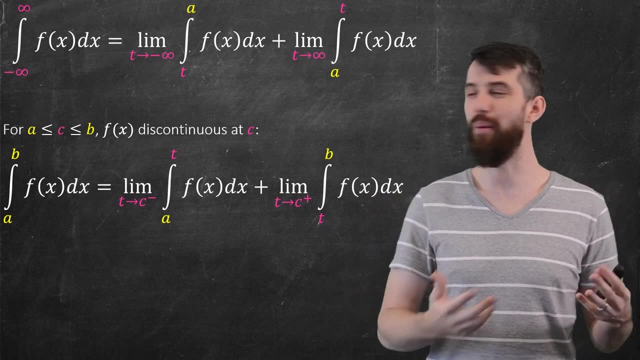 as an integral from a up to t, up to b, and the t values I either send to c from the left or c from the right, depending on which side it is, And then finally you can combine these. you could have a whole bunch of different discontinuities.